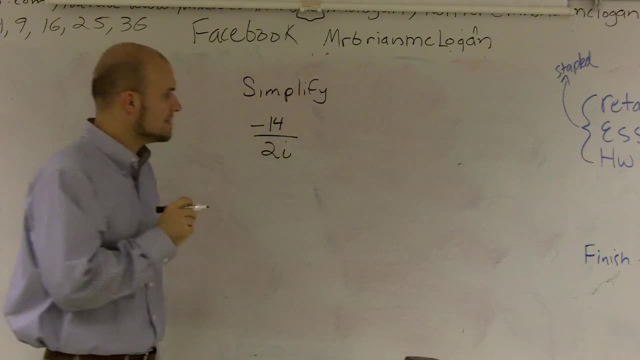 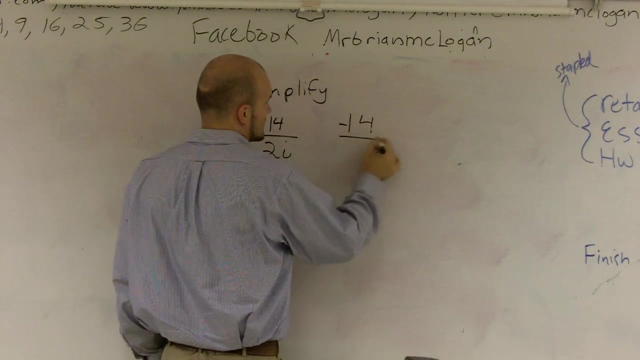 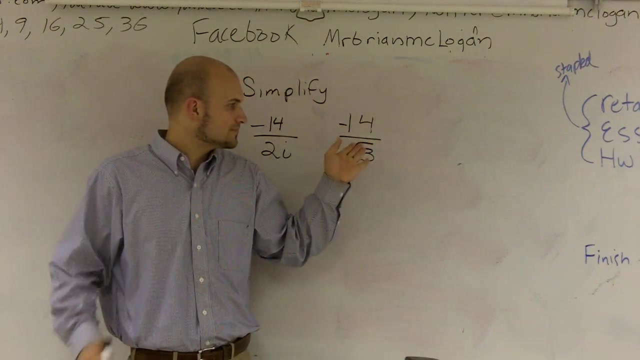 right. And so in our imaginary value, if you can kind of think of it like this, when I had 4 over, let's just do negative 14 over the square root of 3, the square root of 3 goes on forever and ever. right, And you don't know the n to the square root of 3, and it's. 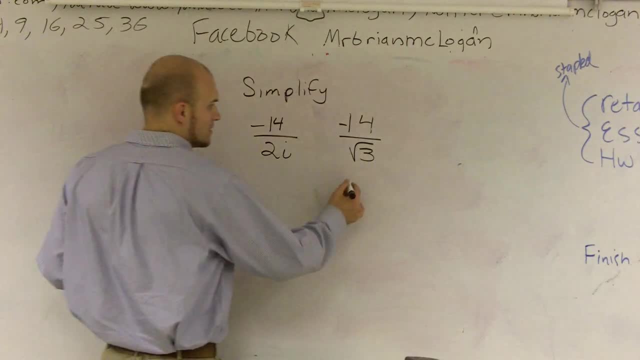 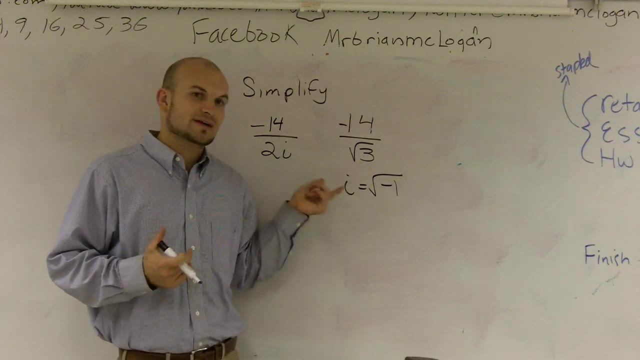 an irrational number. Now, what does i represent? Well, we let i represent the square root of negative 1, because since we can't take the square root of a negative number, we give i the representation of a negative 1.. So, really, you could rewrite this problem and 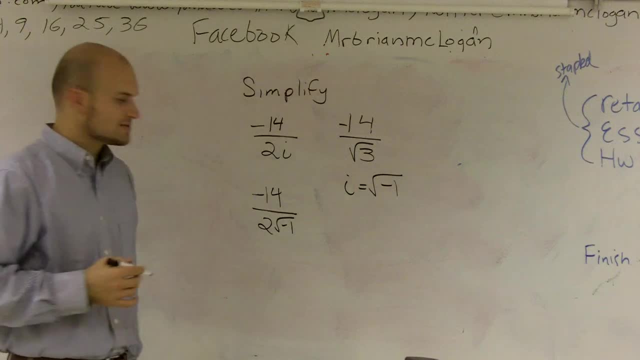 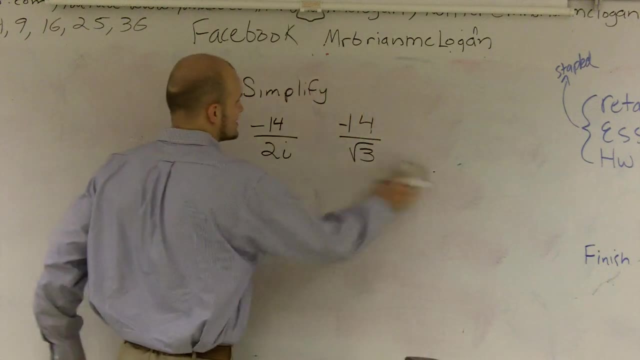 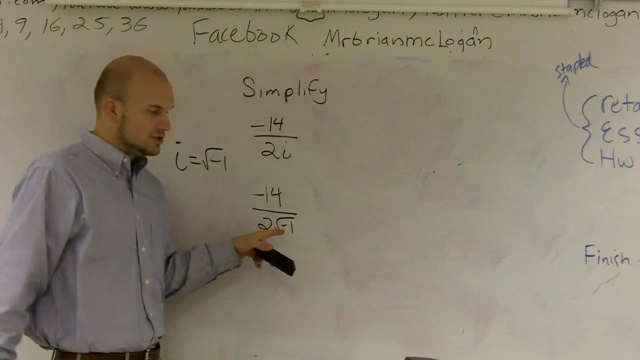 say 2 times the square root of negative 1,, alright, And I'm actually going to do these problems simultaneously together, so you can see that, you know. you know, i is equal to the square root of negative 1.. So if I was to plug these in interchangeably, you should remember that. 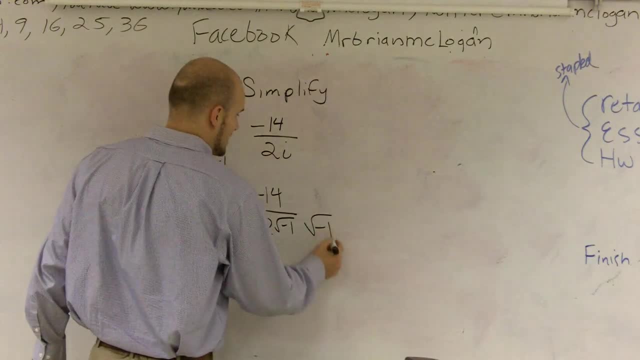 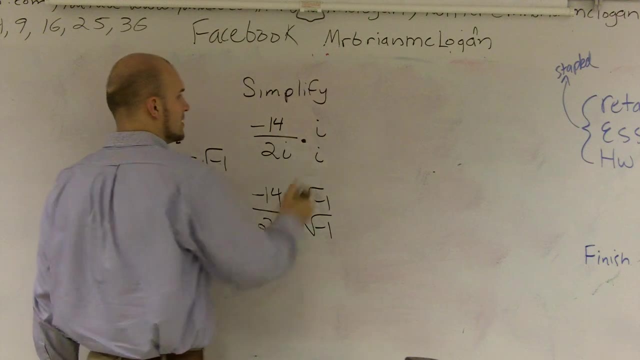 we to do this? we have to rationalize the denominator, which means I'm going to multiply by the square root of negative 1.. Well, similarly, I'm going to multiply here by i over i, and what I obtain is negative 14. i all over 2, i squared. Well, that's what happens here. What happens here? 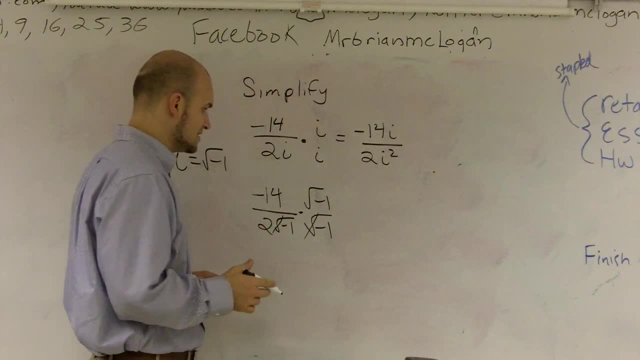 is my square roots. cancel out and I'm left with negative 1 times negative 1, which is a positive 1 times 2.. Yes, So I'm left with- let's see negative 14, negative i and negative. 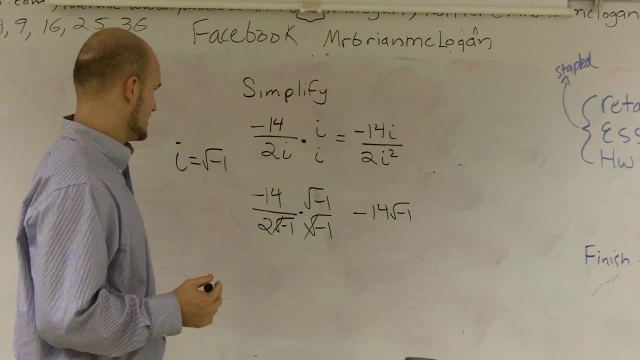 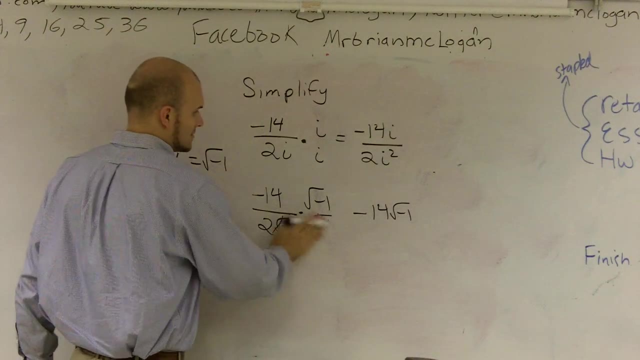 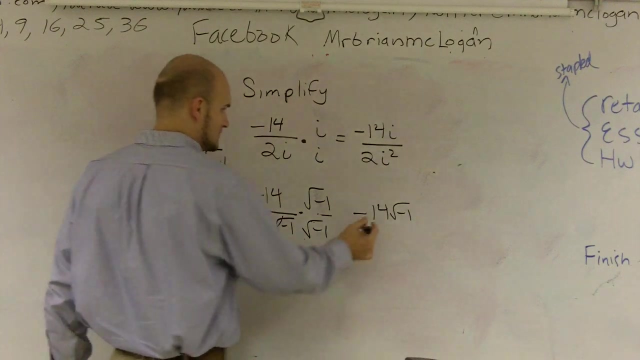 i squared is going to be negative 1.. Oh, I'm sorry that's. I'm sorry that's not going to be squared. This equals 2 times the square root of negative 1 squared. Those cancel out, so you're left with a negative 1.. Negative 1 times 2 gives you a negative 2, alright. 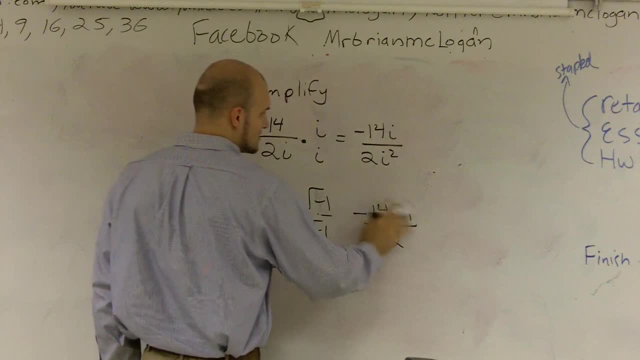 And then, since the square root of i is equal to 1, I can just replace this with an i, And either way, what's going to happen is this is the same thing as negative 14: i all over 2 times negative 1, which that ends up equaling negative 14- i all over a negative.